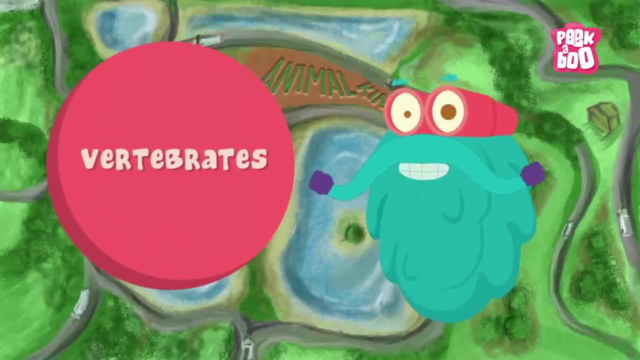 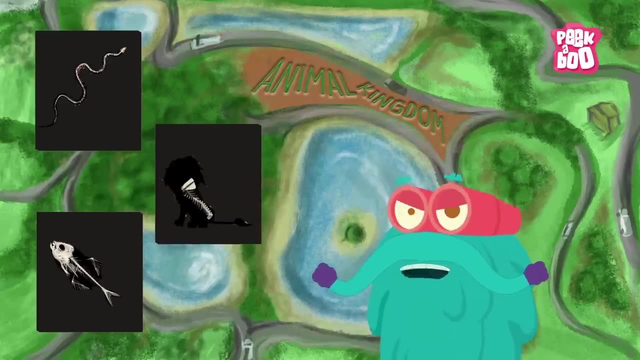 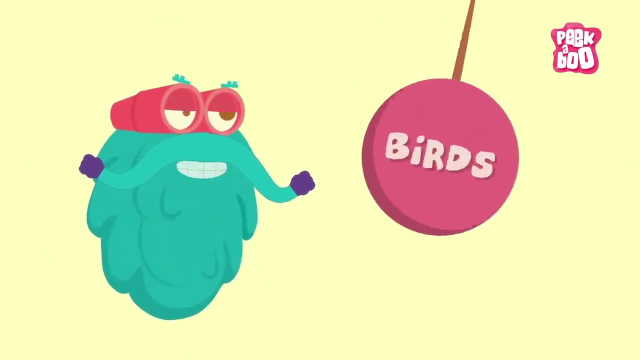 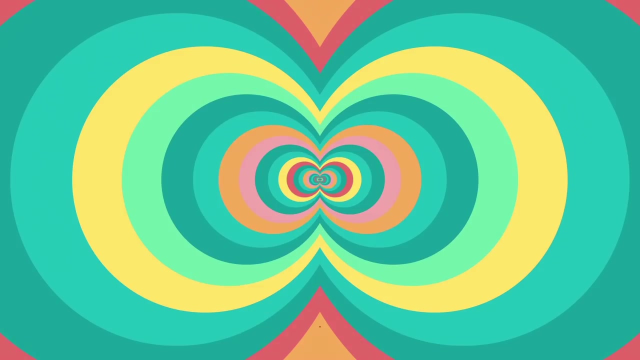 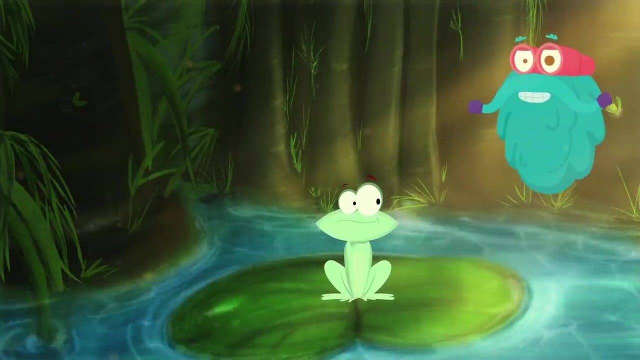 But today we'll talk about the vertebrates. The animals with a backbone are called vertebrates, which are further split into smaller groups: Amphibians, reptiles, birds and mammals. Now let us explore a little into their worlds. Amphibians, Frogs and salamanders are some of the most popular amphibians. 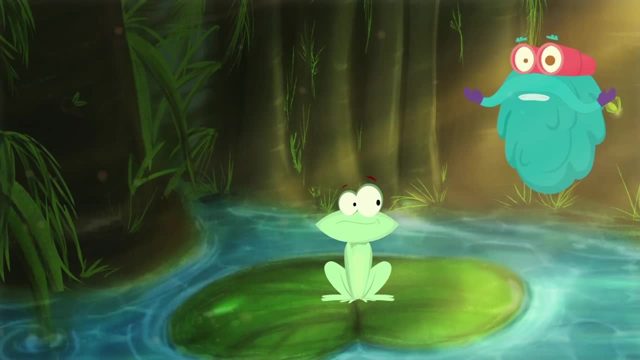 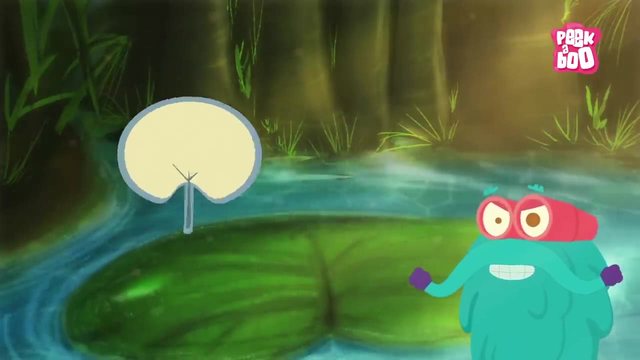 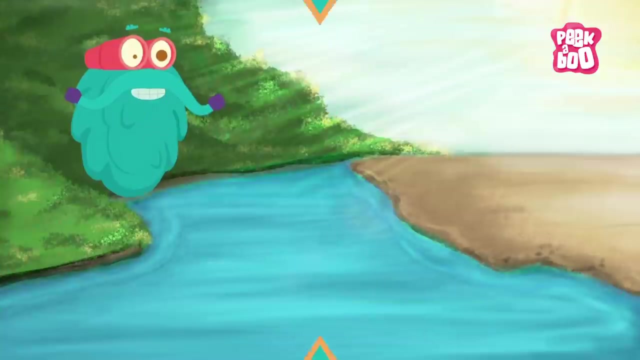 They are the ones that can live both on land and water. They are cold-blooded animals and lay eggs coated in jelly. They have gills to breathe under water and lungs to breathe on land. Reptiles, Snakes and crocodiles are examples of reptiles. 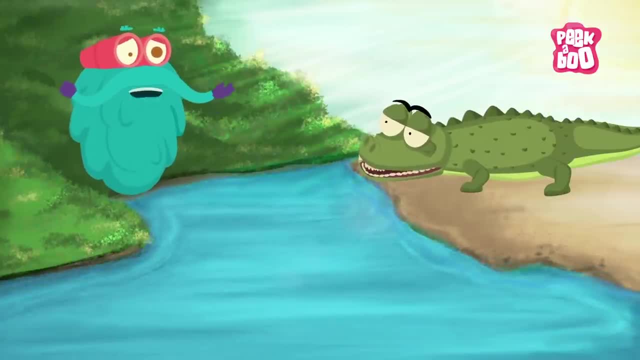 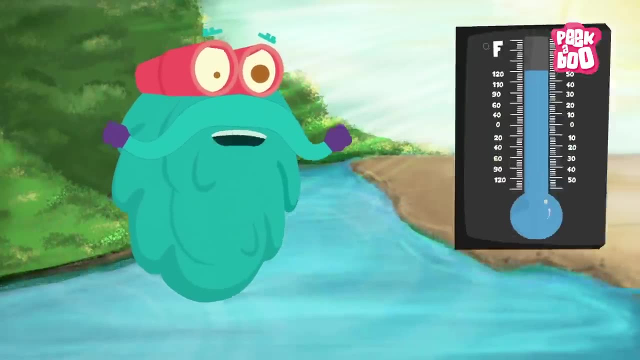 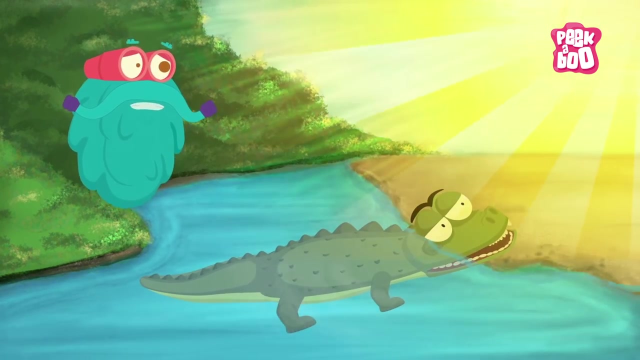 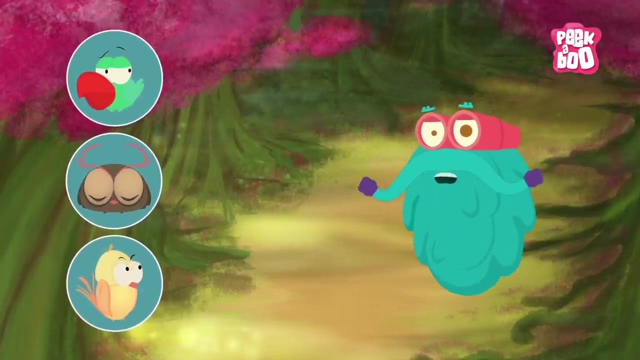 Their bodies are made of dry scales. They lay their eggs on land And spend almost all their time under water. They too are cold-blooded, And it is only sometimes that they come on land to soak the sun. Birds- Oh, you've all seen birds, haven't you? 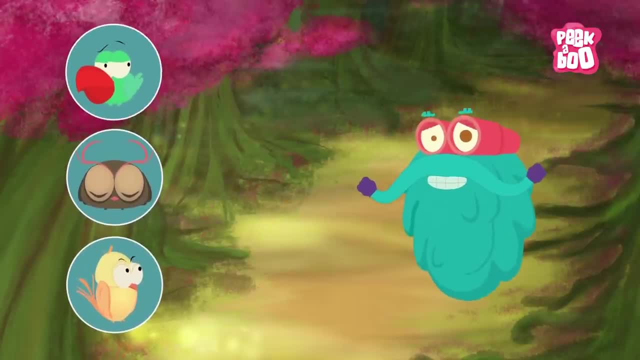 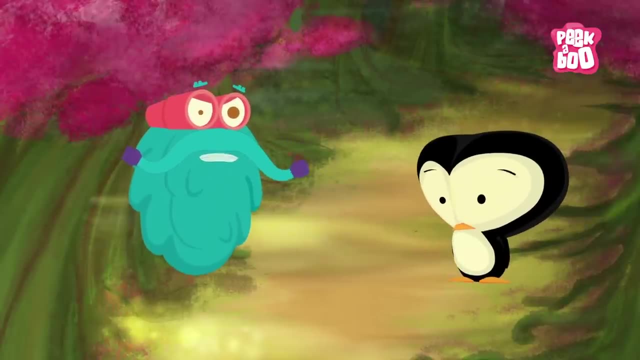 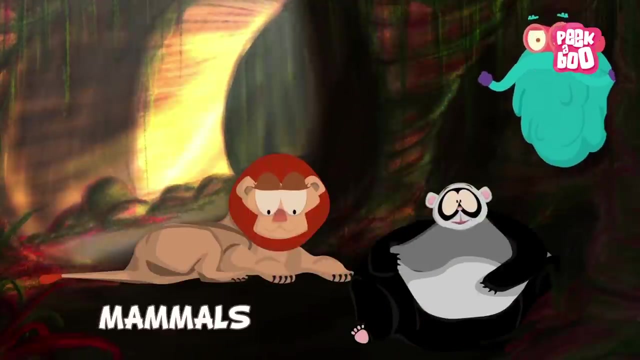 Owls, sparrows, parrots, etc. Well, they have feathers and wings, But hey, Not all birds fly. They lay eggs that are hard-shelled and are warm-blooded Mammals. Lions and pandas are examples of mammals. 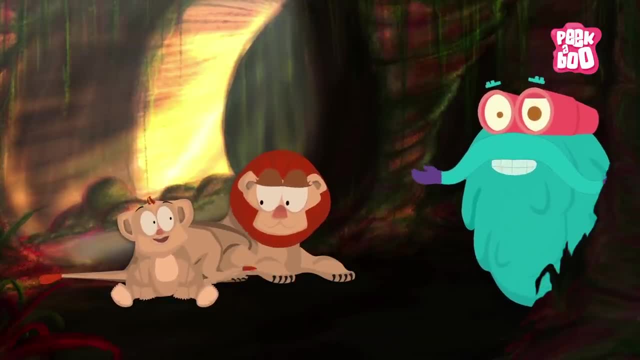 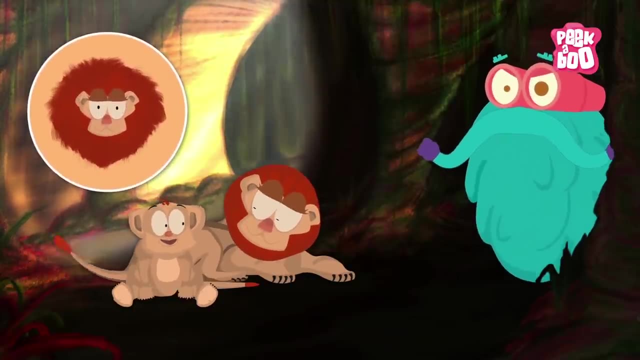 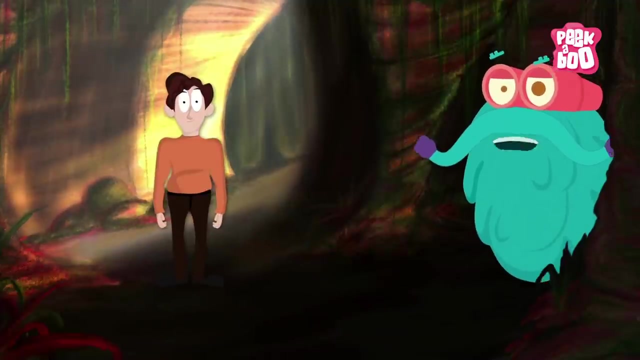 They give birth to young ones instead of laying eggs. They have lungs to breathe and are warm-blooded. They have hair or fur and have special glands to produce milk for the young ones. Even humans are mammals. Yes, you are Trivia time. 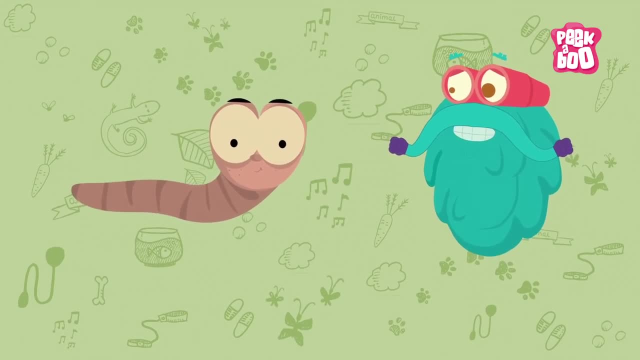 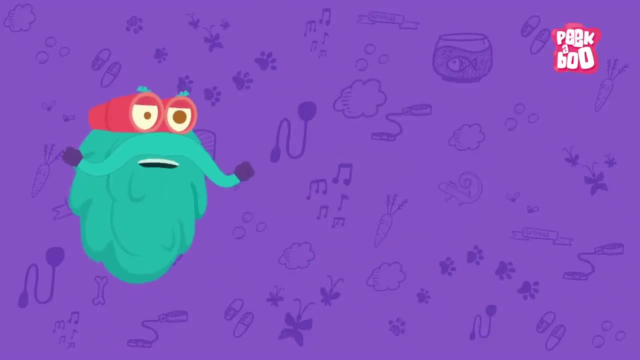 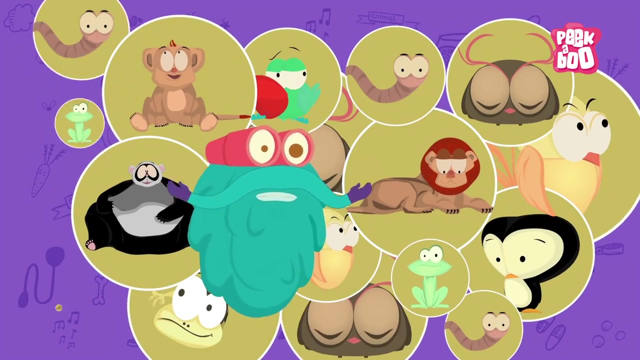 Animals without a backbone are called invertebrates, And they were the first animals to evolve. There are approximately 52,000 species of vertebrates, So what are you waiting for? Look around and start identifying. This is me Zooming out. 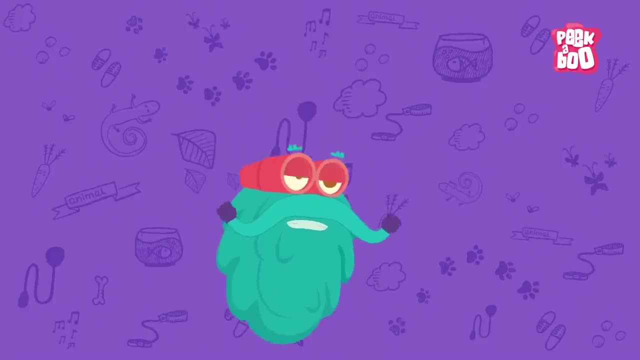 Tune in next time for more fun facts.